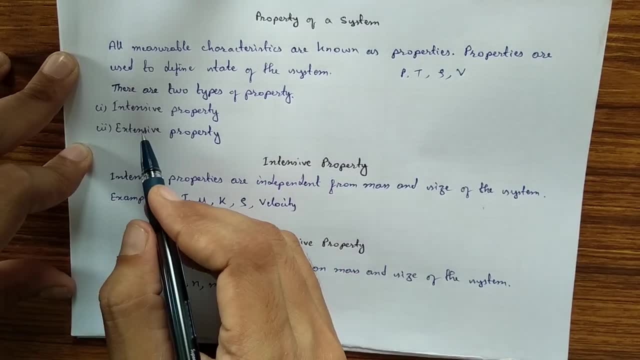 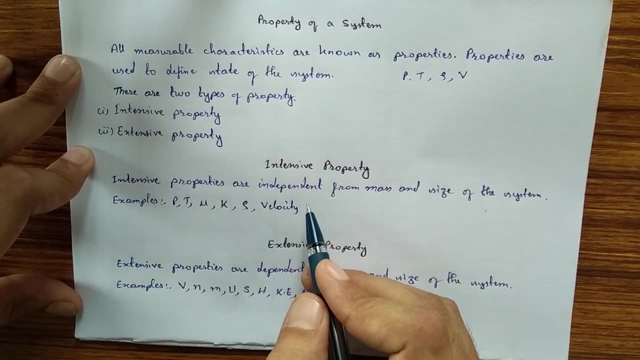 So there are two types of property: intensive property and extensive property. So let's start with intensive property. Intensity property: those properties which are independent from mass and size of the system, that is, they do not depend on the mass and size of the systems. Those 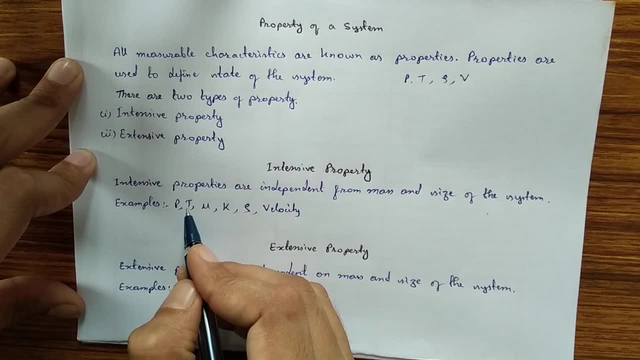 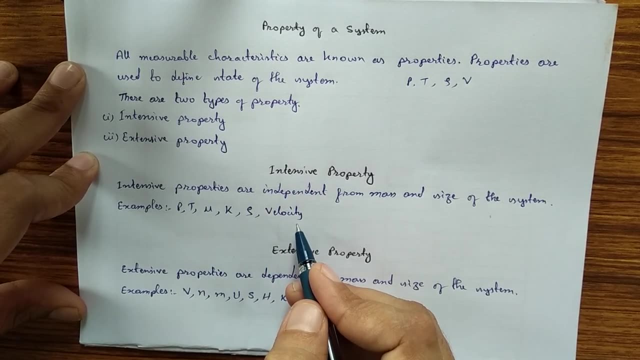 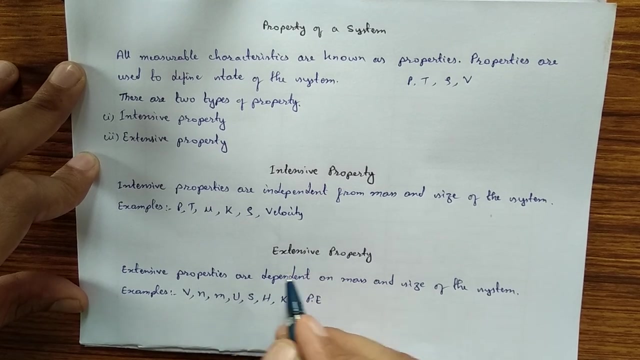 properties are called intensive properties, like pressure, temperature, viscosity, thermal conductivity, density, velocity. These are the properties which doesn't depend on mass and size of the system. Now, extensive property: these are the properties which depend on mass and size of the. 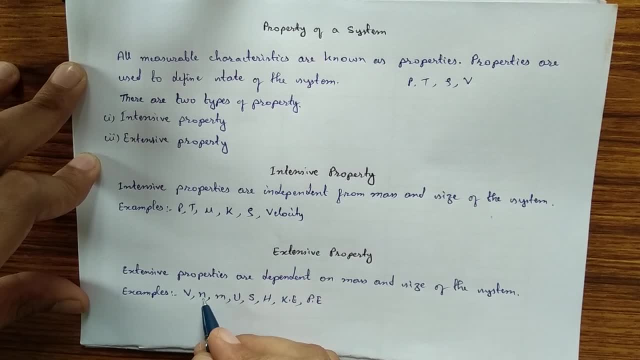 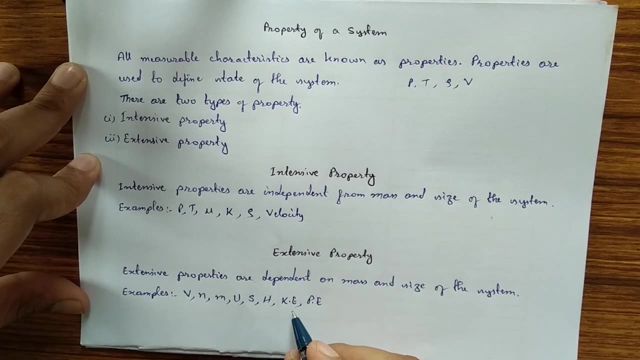 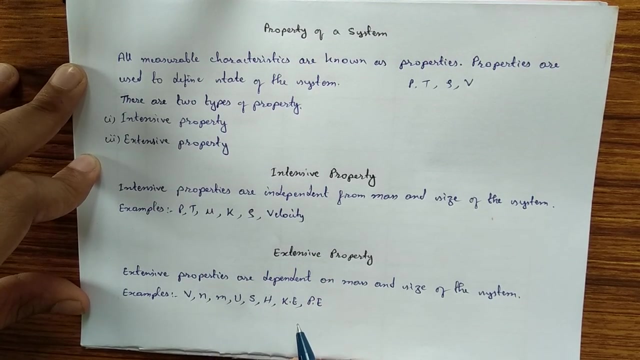 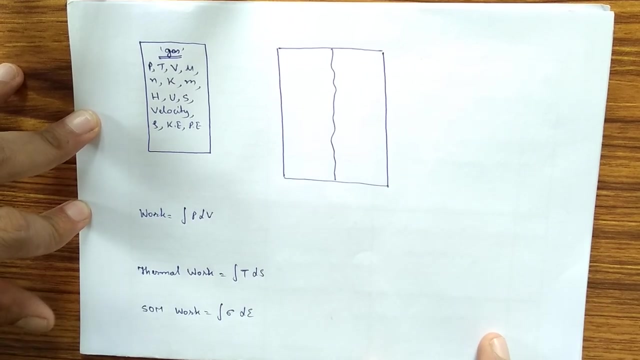 systems, For example, volume, number of moles, mass, internal energy, entropy, enthalpy, kinetic energy, potential, energy. all these depends on mass and size of the system. So these are extensive property. We will better understand these intensive and extensive properties with an example. Let us 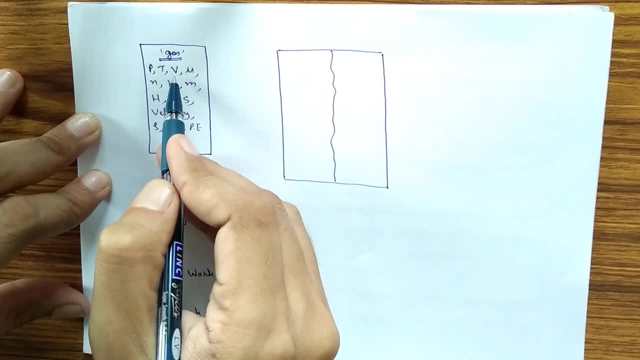 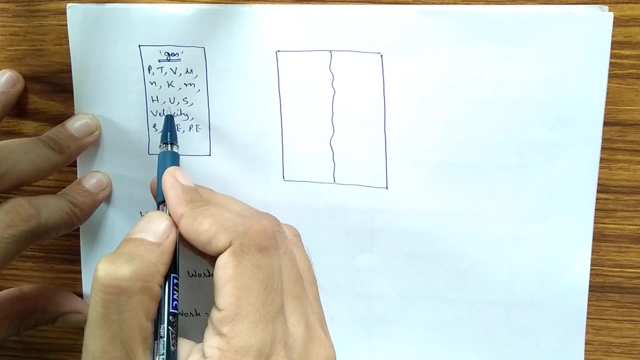 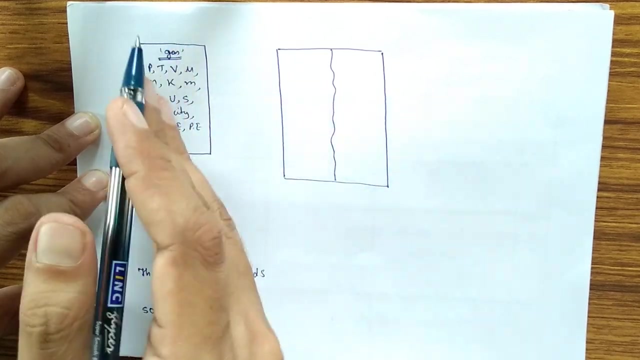 consider a gas in a container whose pressure, temperature, volume, viscosity, number of moles, thermal conductivity, mass enthalpy, internal energy, entropy, velocity, density, kinetic energy, potential energy are given. If we divide this container into two parts, say A and B, then 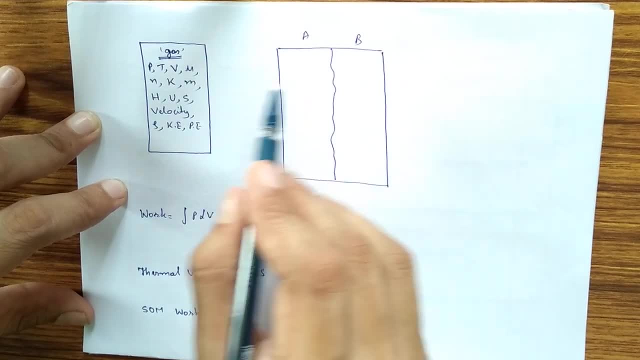 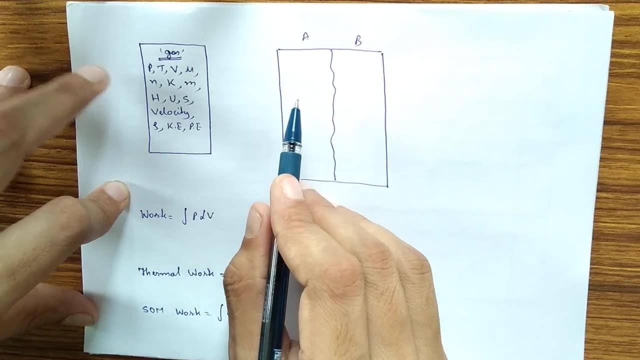 we will see what are the properties which gets divided. Those properties which gets divided will be considered extensive property and those which is not divided is intensive property. So see pressure. If we divide the container into two parts, then pressure will remain same in both. 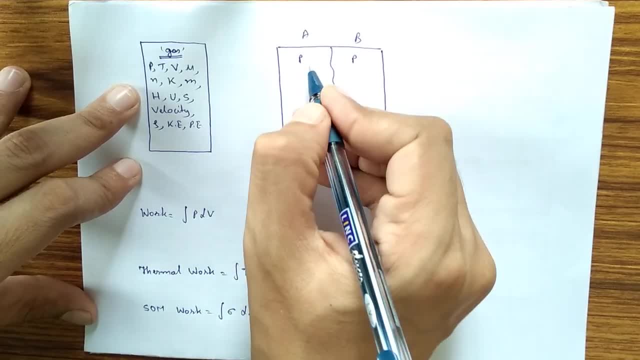 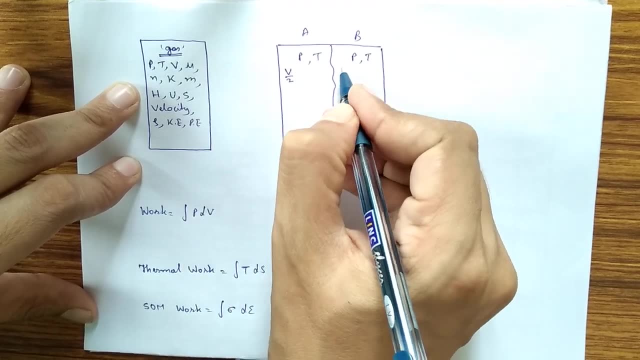 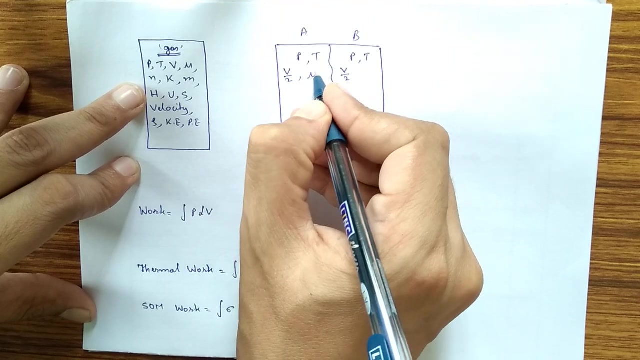 the parts, So it is an intensive property. Temperature will also be the same in both the parts. Volume volume gets half, So it is an intensive property. So it is an intensive property, Extensive property. viscosity: it will remain same. It is an intensive property. Number of: 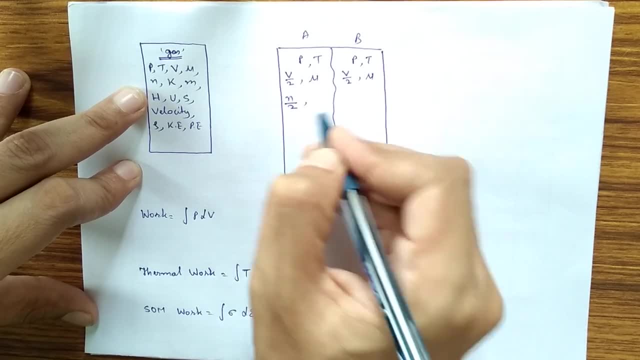 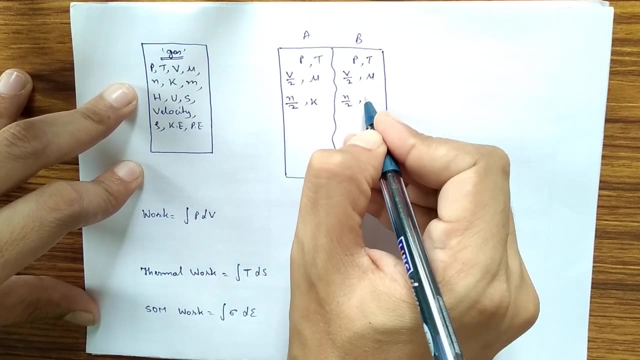 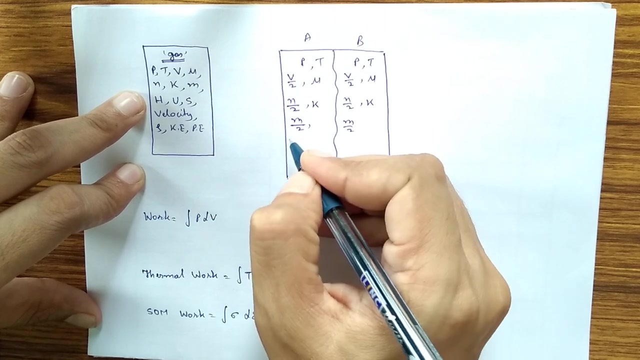 moles: it will get half, So it is an extensive property. Thermal conductivity: it will be the same, So it is an intensive property. Mass: it will get half, So it is an extensive property. Enthalpy: it will also get half, So it is an extensive property. 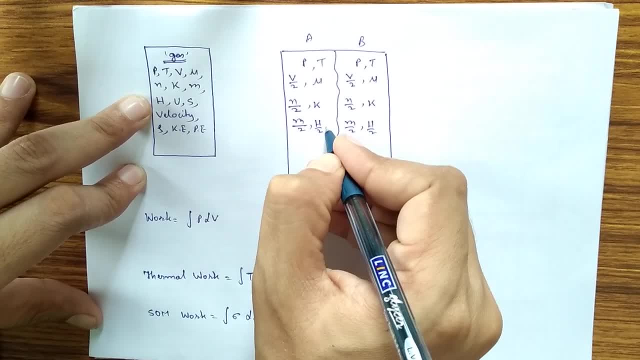 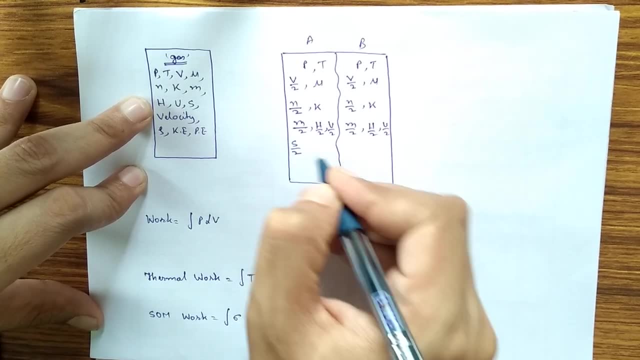 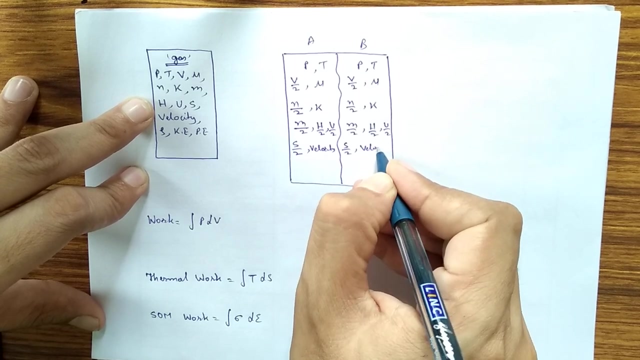 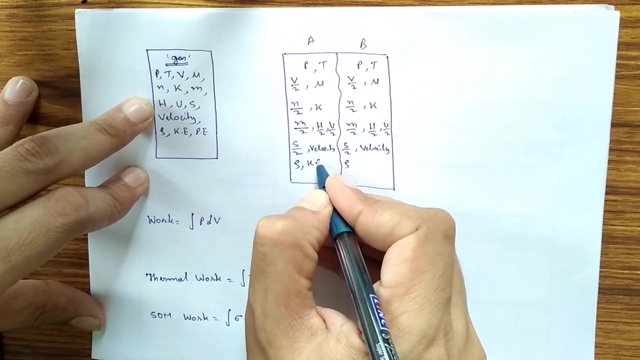 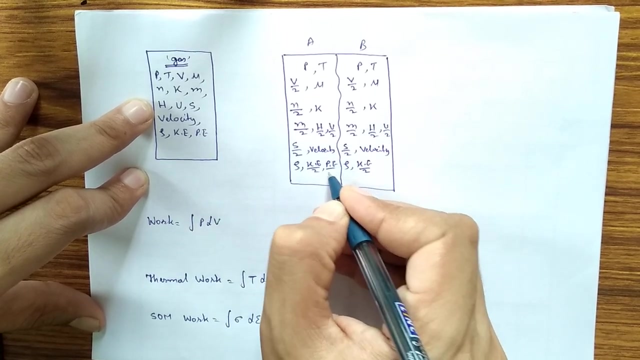 half. internal energy will also get half entropy: it will also get half. velocity will remain same, so velocity is an intensive property. density will remain same, so density is an intensive property. kinetic energy will be half, so kinetic energy is an extensive property. potential energy will also become half. 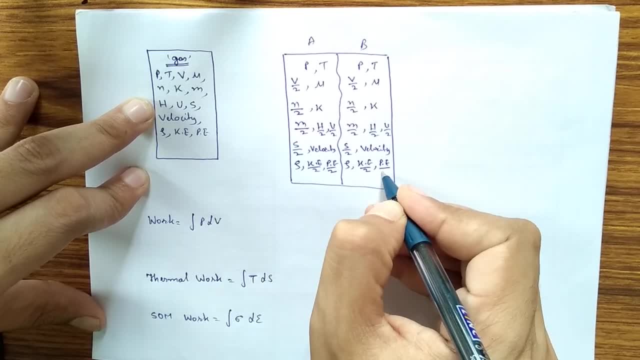 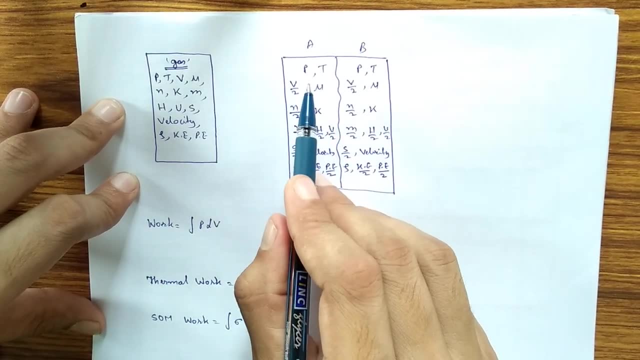 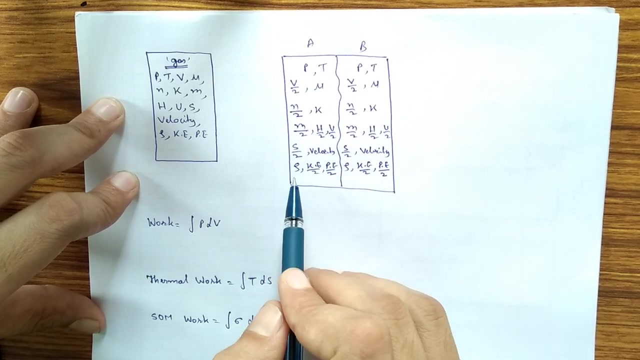 so this is also an extensive property. so whatever the property we see here which doesnt get divided, those all are intensive property, like pressure, temperature, viscosity, thermal conductivity, velocity, density. these all are intensive property. and those properties which gets divided are like volume, number of moles, mass, enthalpy, entropy, enthalpy internal energy entropy. 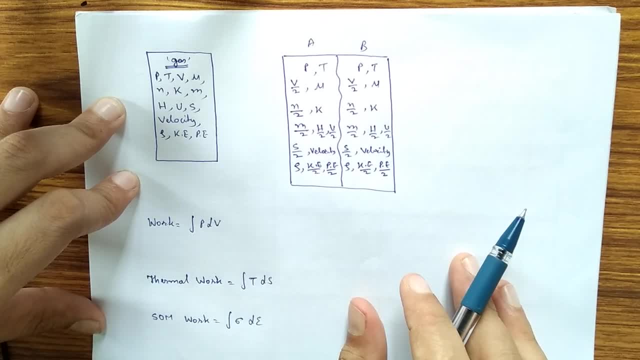 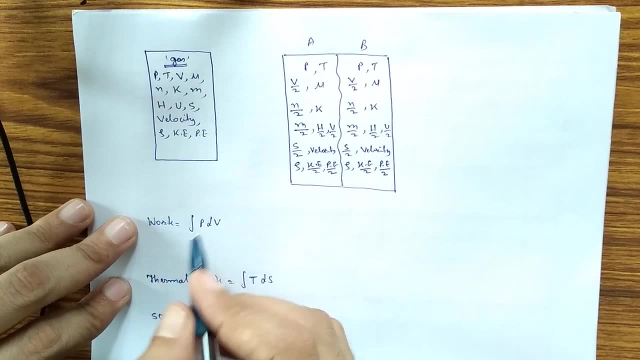 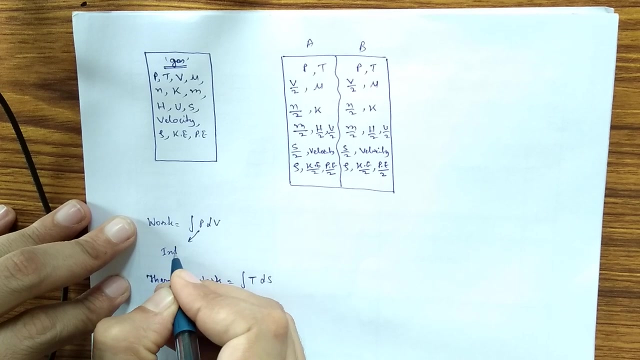 kinetic energy, potential energy, these all are extensive property. so if we see the expression of work, so in the first we'll see the pdv work, where p is the pressure and dv is the change in volume. in the expression of work first one is intensive property and the other one is 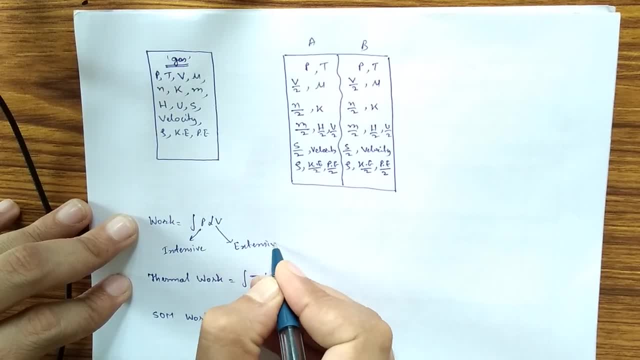 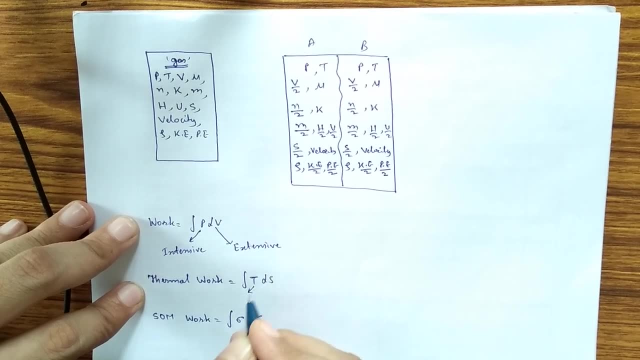 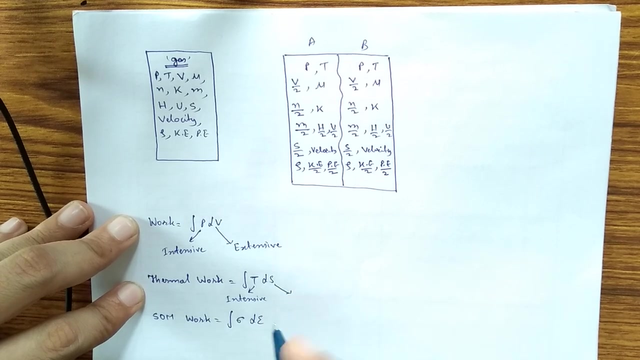 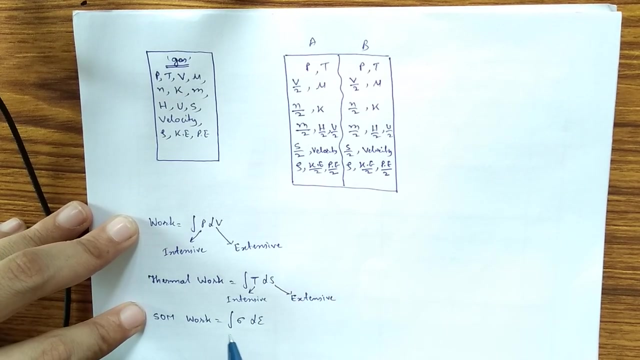 extensive property. if you see thermal work, tds work- where t is the temperature and d is the change in entropy. so temperature is the intensive property and in change, entropy is the extensive property. in some work, integration of sigma d e epsilon- sorry, sigma epsilon, where sigma is the 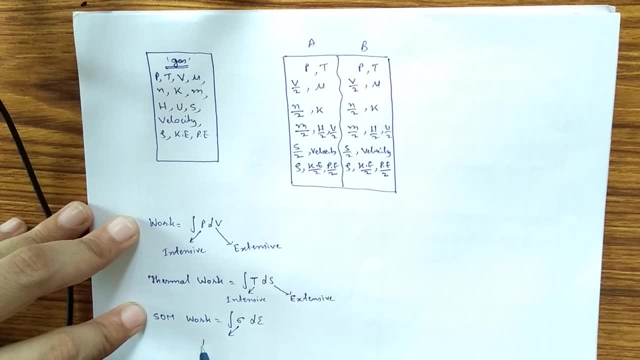 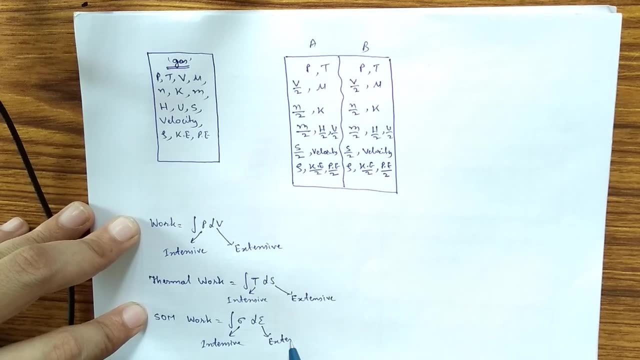 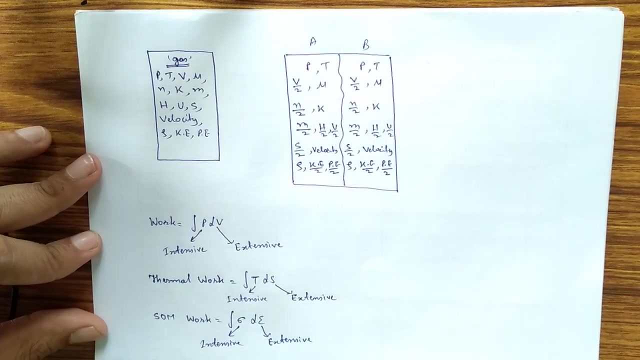 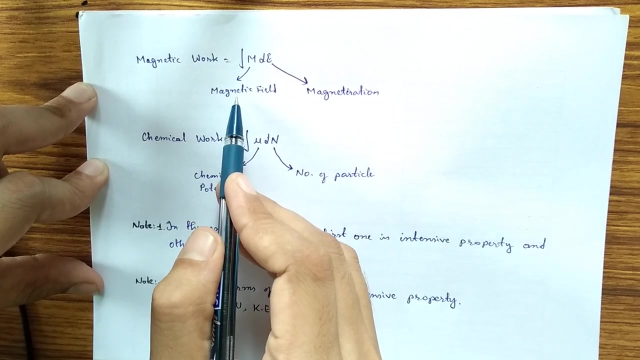 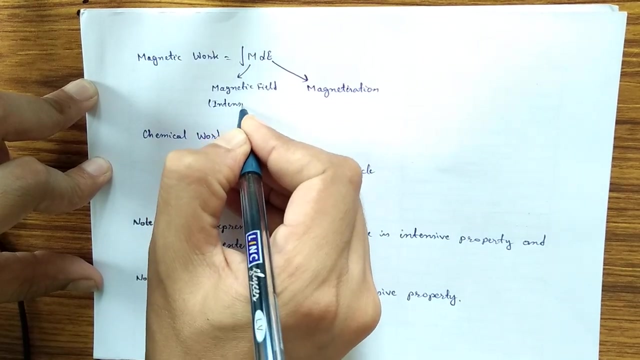 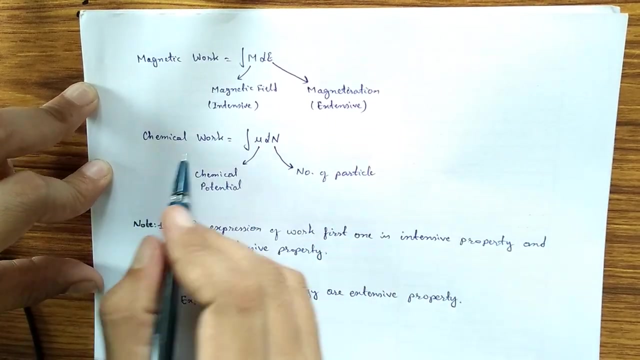 stress and epsilon is the strain. so this is intensive and this is extensive. if we see magnetic work, integration of mde, where m is the magnetic field and d is the magnetization, so this is intensive property and this is extensive property. if we see chemical work integration of mu- dn, where mu is the chemical potential, 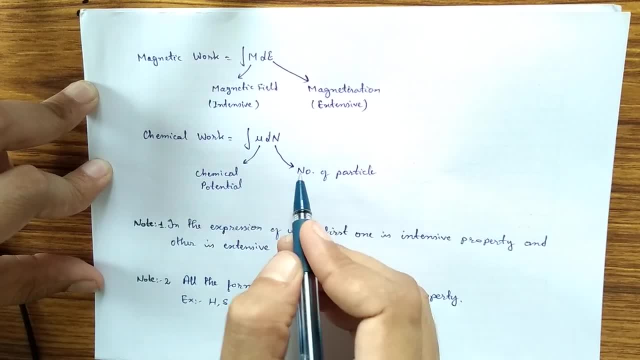 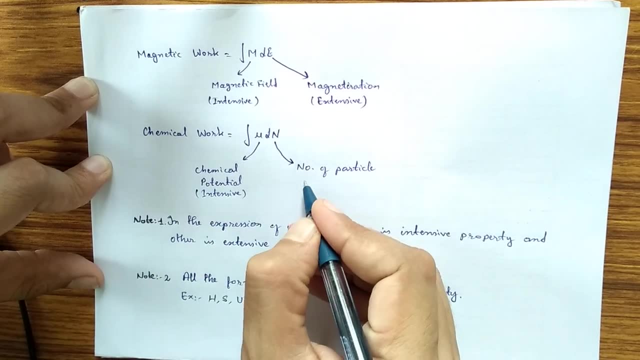 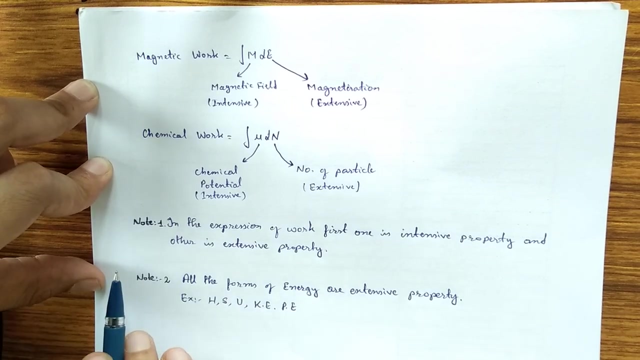 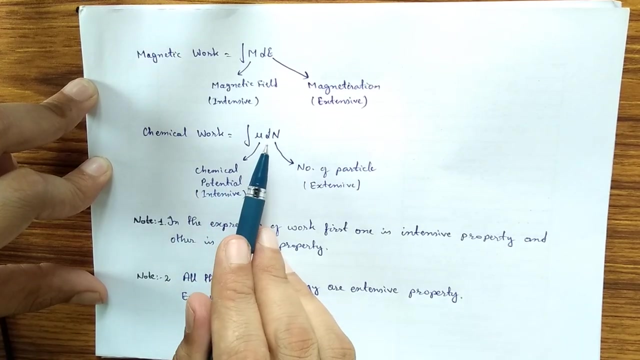 and dn is the number of particles. so this is intensive and this is extensive. so one thing can be noted: that in the expression of work we see that the chemical work is very extensive. in the expression of work, first one is intensive property and the other one is extensive property. 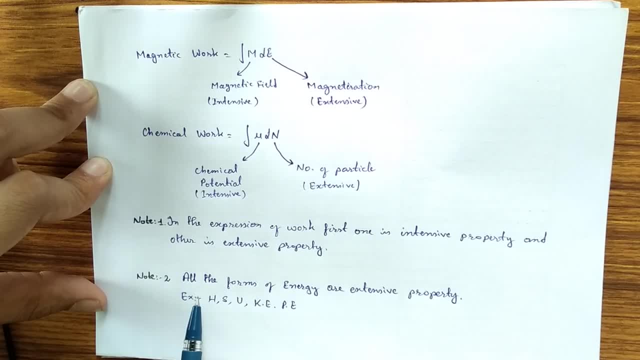 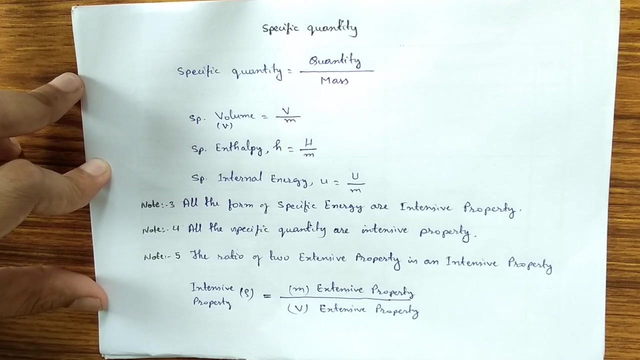 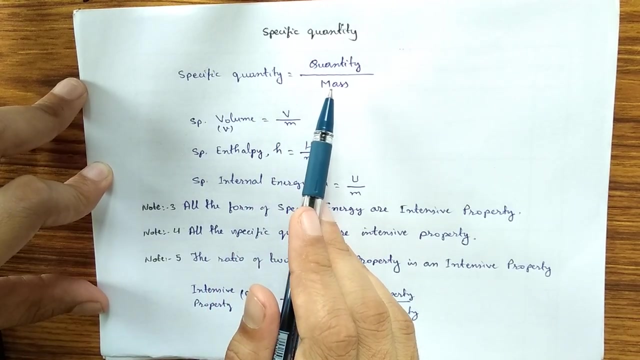 also we can see, no, we can note that all the forms of energy are extensive property, like enthalpy, entropy, internal energy, kinetic energy, potential energy. so all the forms of energy are extensive property. specific quantity. so what is specific quantity? quantity per unit mass is called a specific. 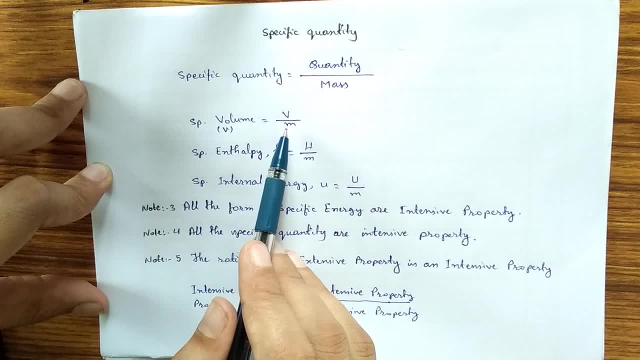 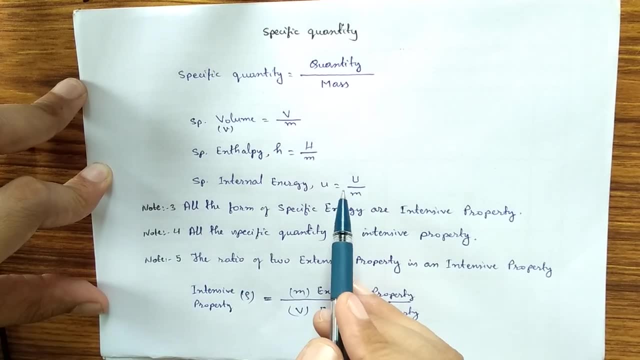 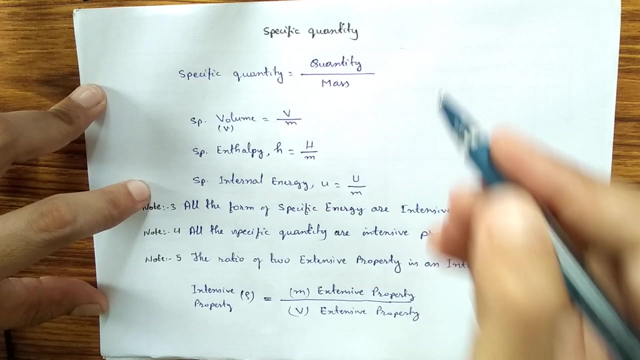 quantity. example: a specific volume: volume per unit mass. specific enthalpy, which is denoted by small h: enthalpy per unit mass. specific internal energy: internal energy per unit mass. so all the form of specific, specific energy are intensive property. we can take an example like kinetic. 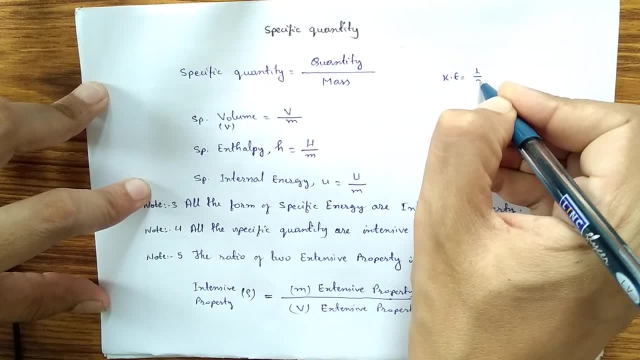 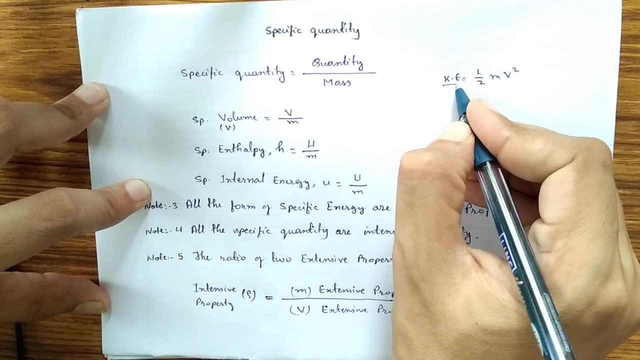 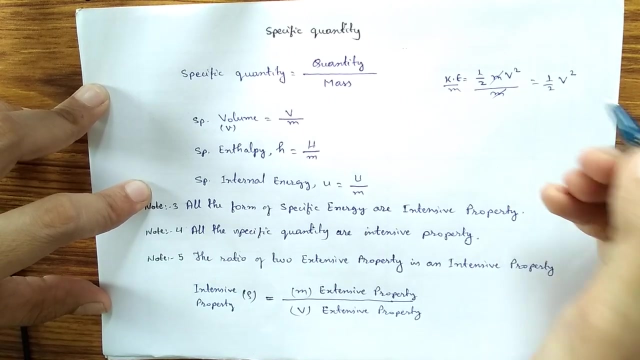 energy. it's expression is half mv square. so if we consider as specific kinetic energy, we will divide it by mass. so mass gets cancelled. so it only depends on velocity, which is an intensive property. so specific kinetic energy is an intensive property. so all the form of specific 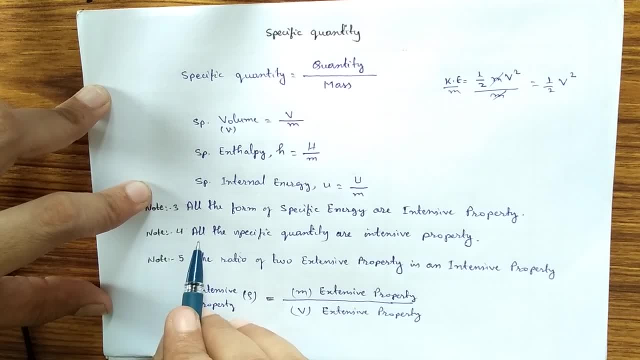 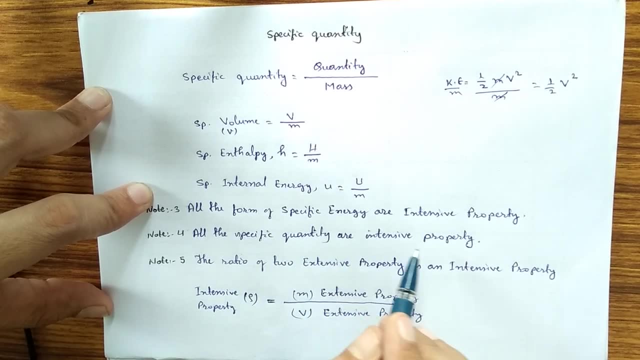 energy are intensive property. also we can note that all the specific quantity are intensive property. so whatever is specific quantity is intensive property. so all the form of specific energy are intensive property. so whatever the specific quantity we are having, so all those quantities are intensive property. the ratio of two extensive property is an intensive property. 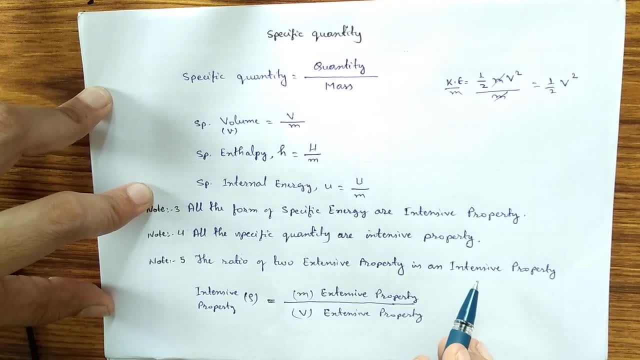 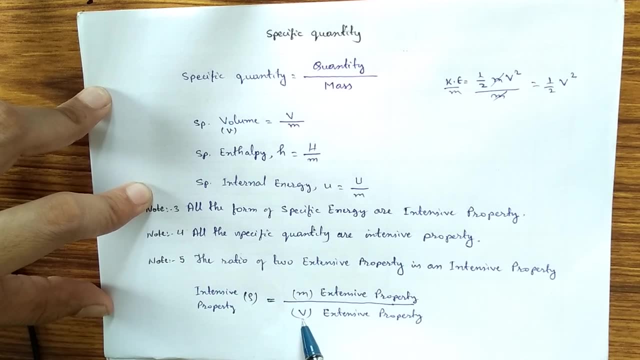 so if we take the ratio of two extensive property, we will get an intensive property, for example, density, which is a ratio of mass by volume. so mass is an extensive property and volume is also an extensive property. so it is the ratio of two extensive property which is an intensive property. 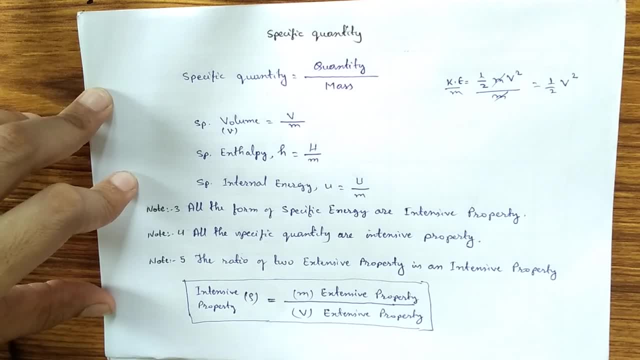 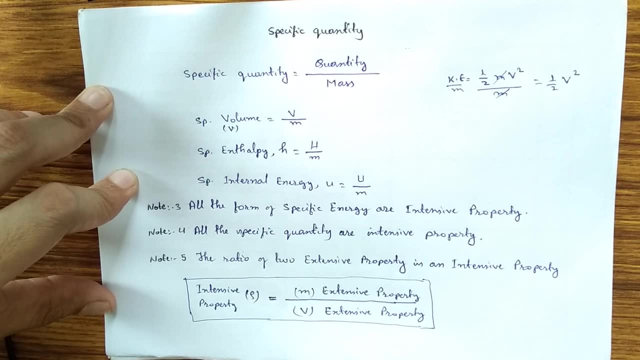 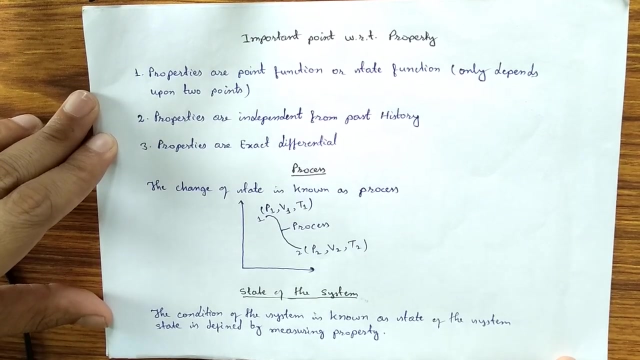 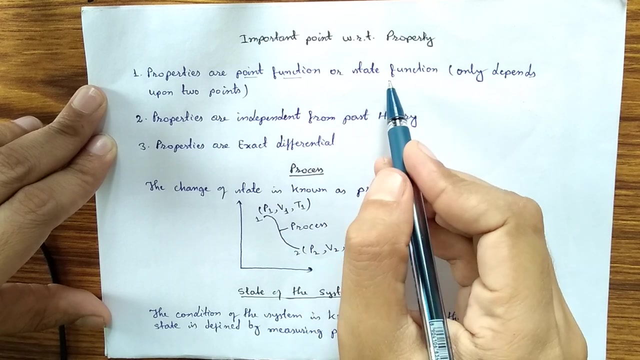 so all the forms of specific energy are intensive property, all the specific quantity are intensive property and the ratio of two extensive property is an intensive property. now important point with respect to property properties are point function, that is, it depends on the point only, or state function only, depends upon two points. so it doesn't depend on the path, it depends on the 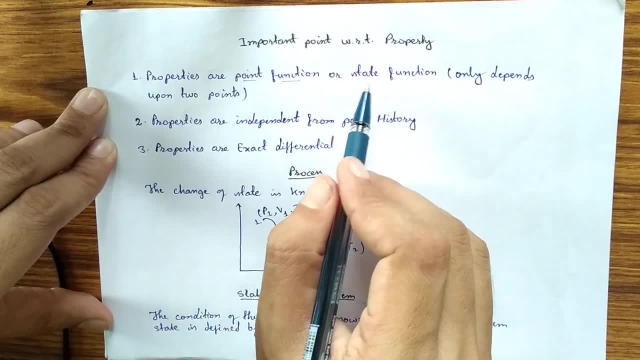 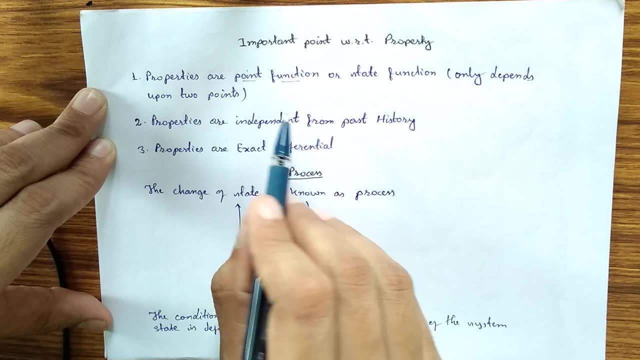 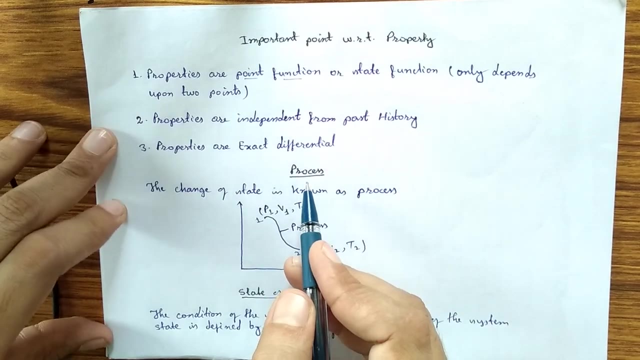 point only. so properties are point function or state function depends upon two points: properties properties are independent from past history. it doesn't depend on the past history. it only depends on the two points. properties are exact differentials, process. so the change of state is known as process. state means the condition of this, the condition of 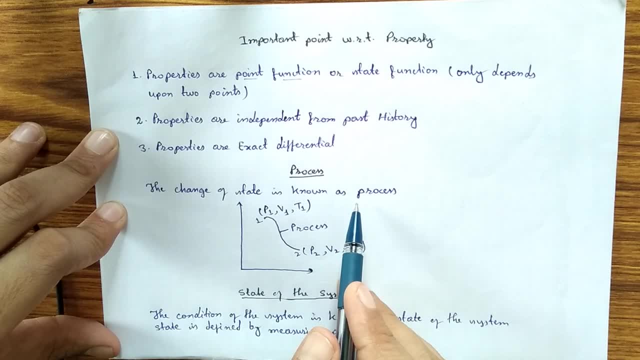 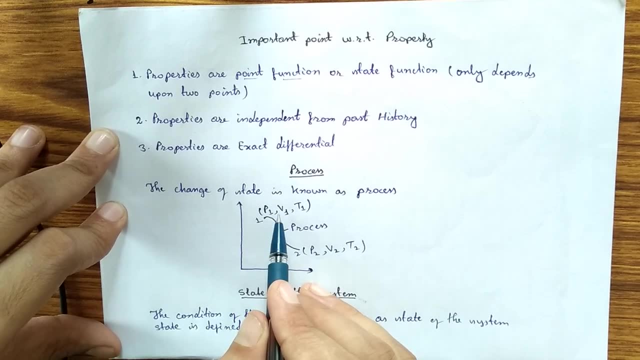 the system is called state, so the change of the state is known as property. so let us consider this results. it is still in product, so we know this one is our process state, so it should be belong to this particular state. it should be prayed there already, okay, so this is in object. 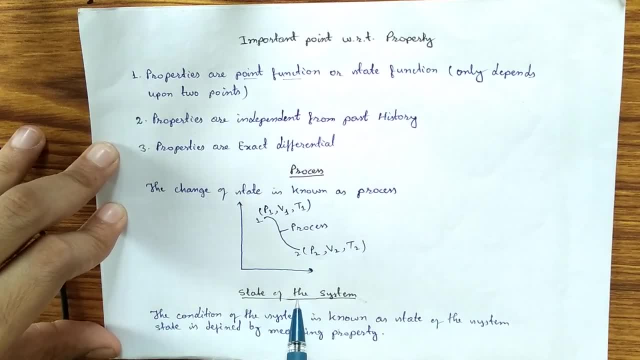 so we need to know this is the kind of state of the system. so we need to know the loss experiences too. so we need to know that all conditions which happen with each one of these properties, because, in fact, if we enter the type, change in the temperatureいて objects can be change. 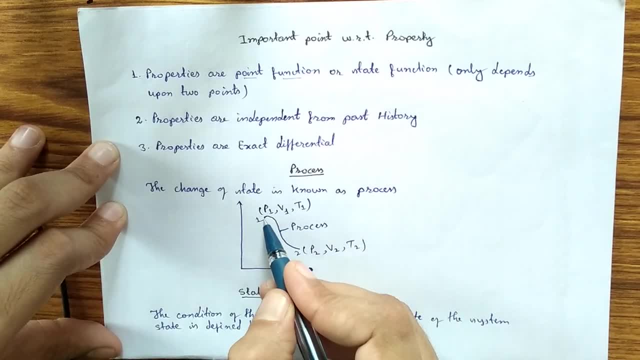 and quindi we have to do also move on to the whole point. i'm not going to explain how there are different issues, which are there significant problems and such thing to do now. we have to go beyond the state of empty spaces because in fact the down to 10 in the bardzo condition state 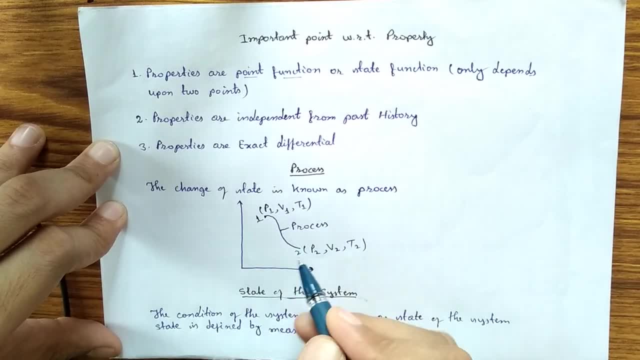 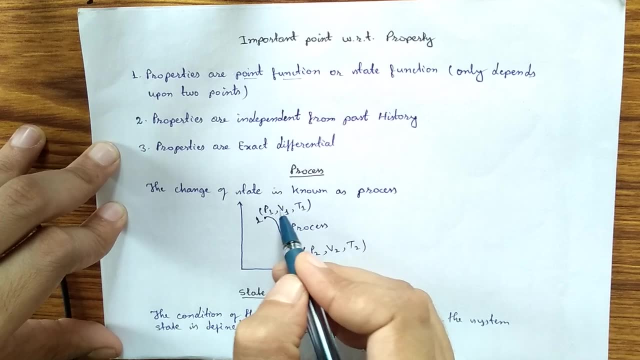 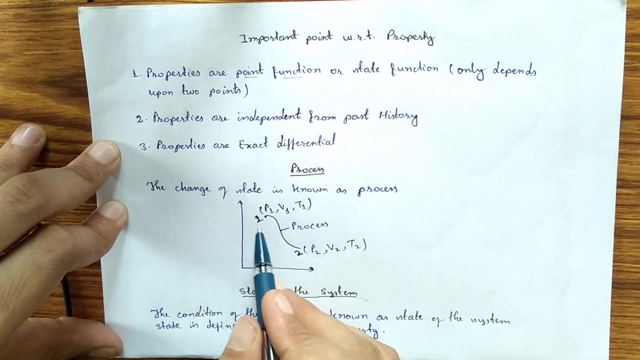 measuring the property. see, this is the one state one and this is state two. we know this is state just by measuring the property, like pressure, volume, temperature of. after knowing these properties, we get to know the state. so, after measuring these properties, we get to know the state and if we change the